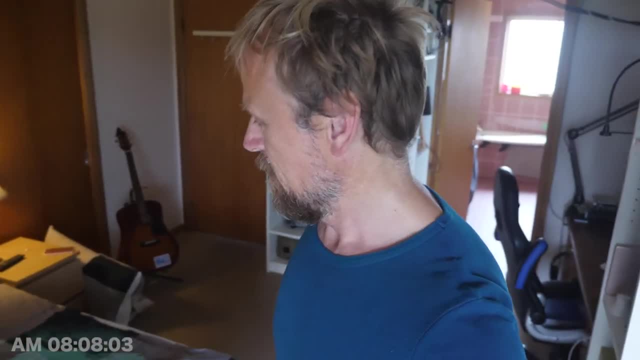 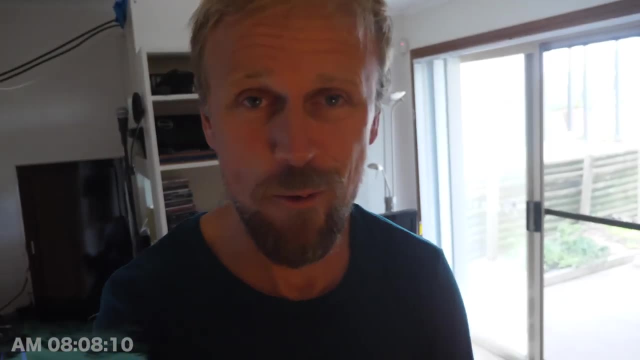 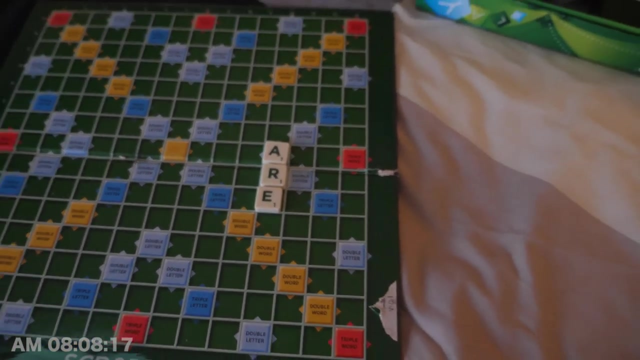 It's 8 past 8.. Good morning. Genuine Scrabble question. right, I've had Marty and Stacey down here playing Scrabble with me and it raised a question I want to ask the givers. So look, let's just say, for example, this word's on the board are. We all know I can play here to make. 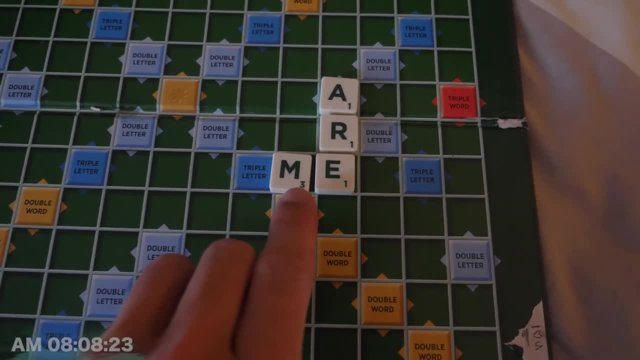 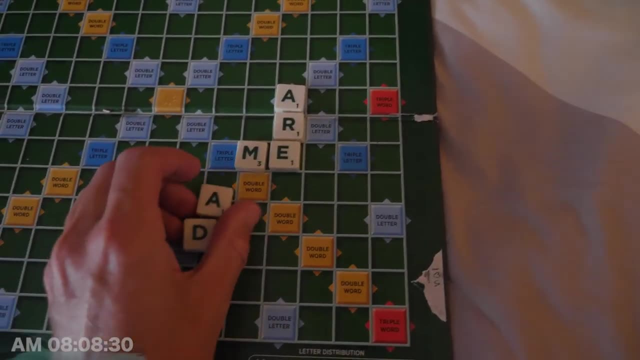 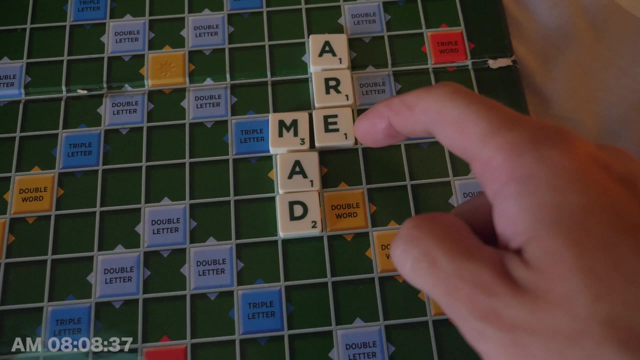 the word me: right, And I get me. Now I could also play a word down here, off the So I could play a word such as mad: right, I'd get the score of mad, and the score of me right, So you'd get. 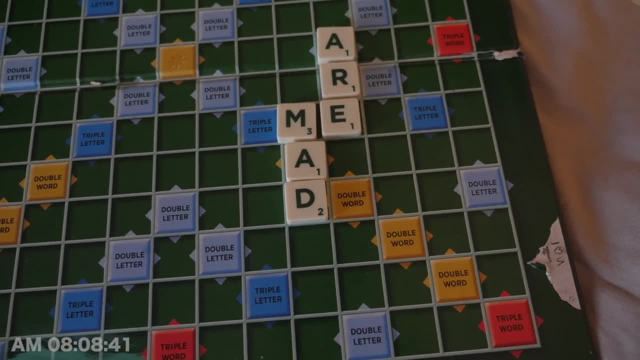 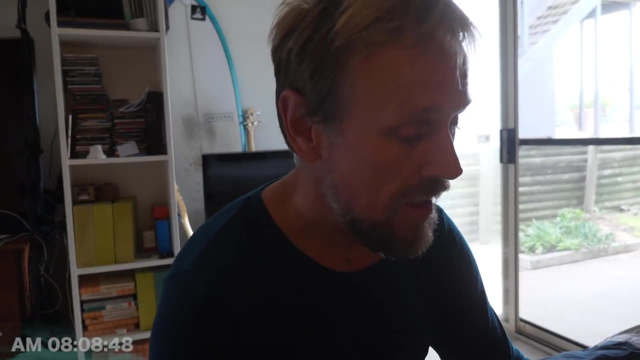 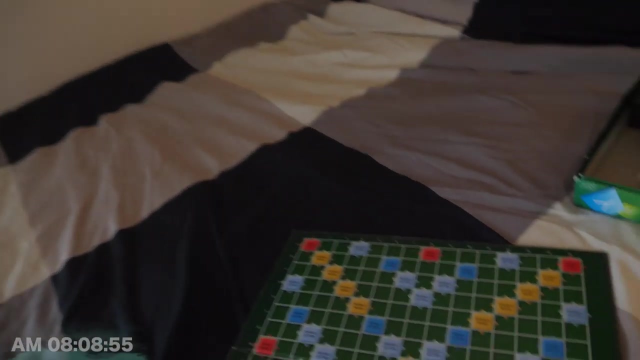 an across score and a down score. The question that came up during the game was: is it possible to get the across score and the down score if the across score is more than two tiles? So an example would be, instead of me playing mad down like this: 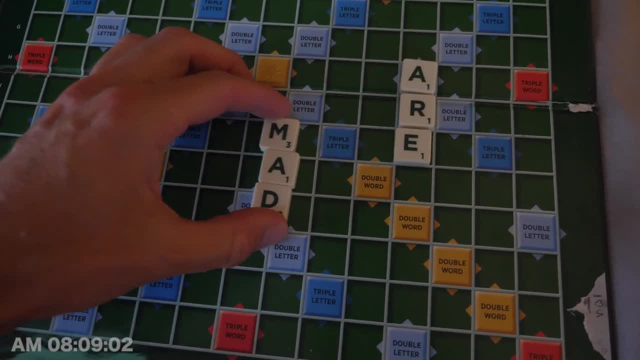 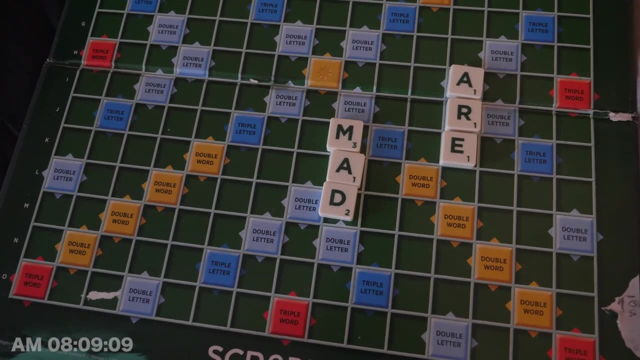 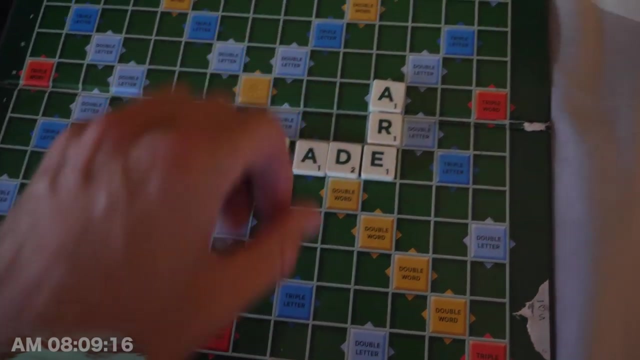 I would put my M over here And so it would still say mad, but obviously you've got to join those up, right? So I'd have to go. I could even go like this: I could go a different word, I could go made, and then I could do the M going off here with more. 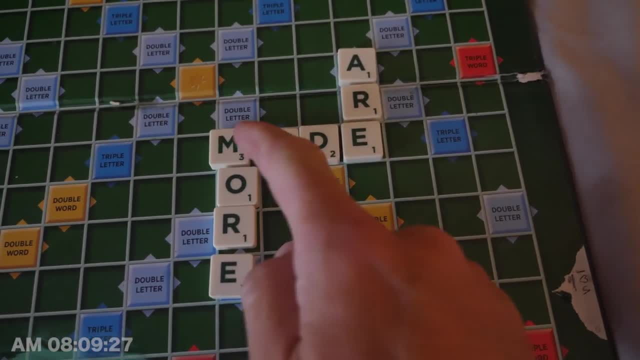 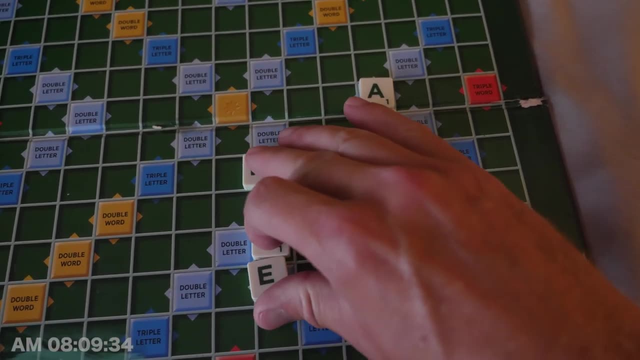 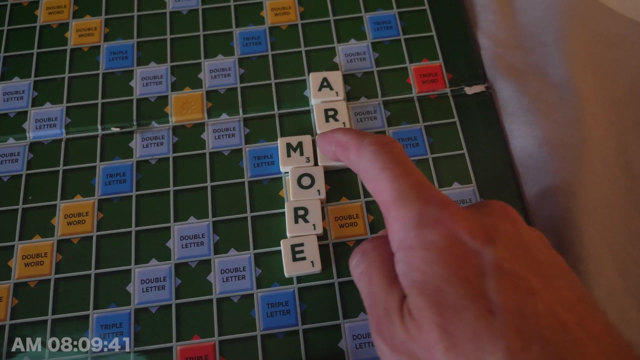 So is that a play that I can do? I can play across to make made and down to make more, Because we were saying that, no, you can only play down here and make this word and it just coincidentally makes this word, And I was saying, that doesn't. 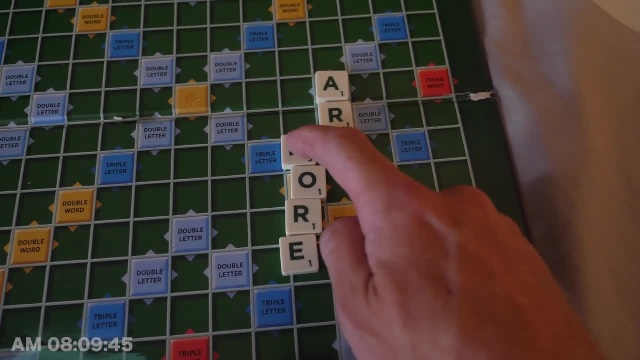 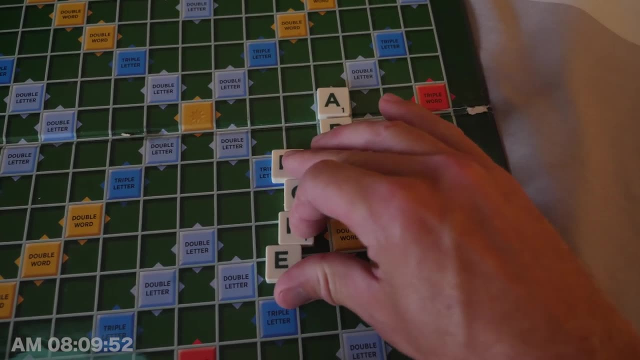 make much sense, because you're only saying I can only have that word if it's a two-letter word. I'm making the word me and I'm making the word more, And in this case I'm making the word made to make the E. 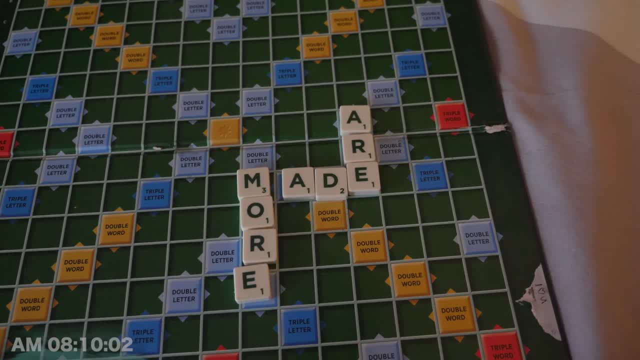 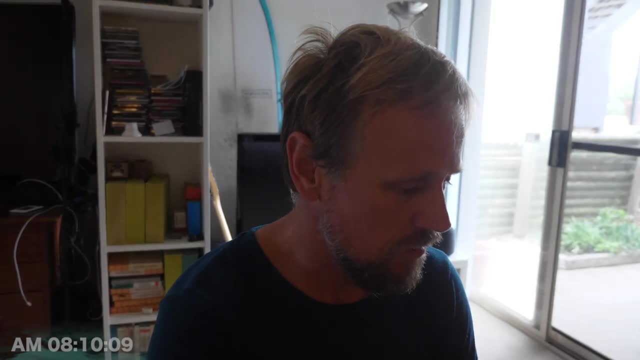 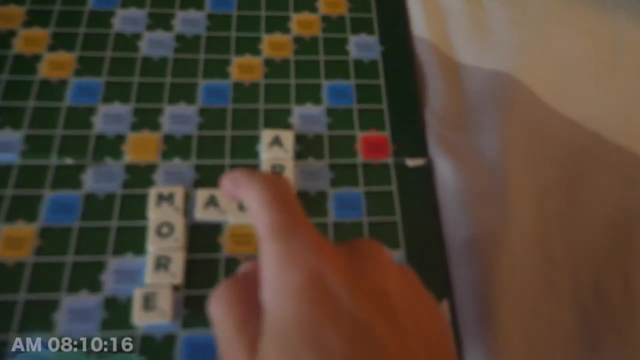 and I'm making the word more. And the question was: well, no, you can't play two directions. You can't play horizontal and vertical. It's like: well, either you can't entirely or you can't Like. if you can't do that, if you can't play,